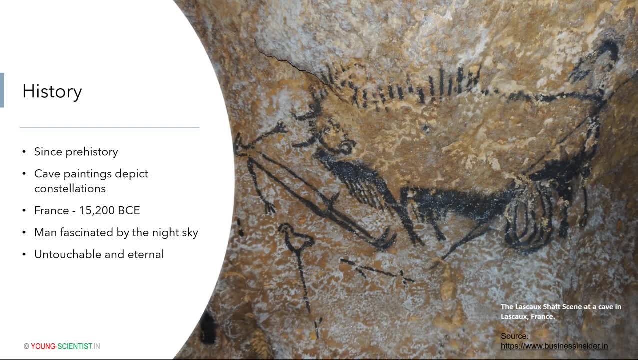 This means that humans have a fundamental fascination to the night sky. Humans have a fundamental fascination to the night sky. What could be the reason? Maybe it is because the night sky is separate from what happens on the planet. We can interact with plants, animals, other humans and we can change things here. 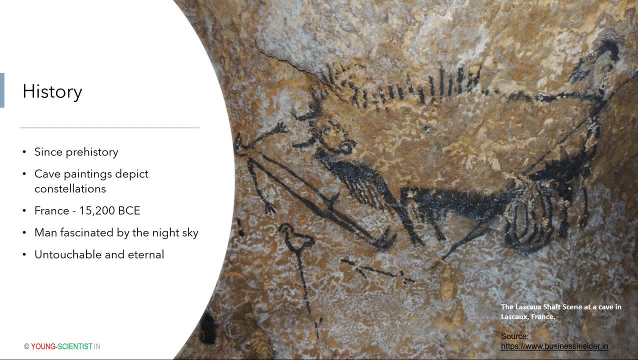 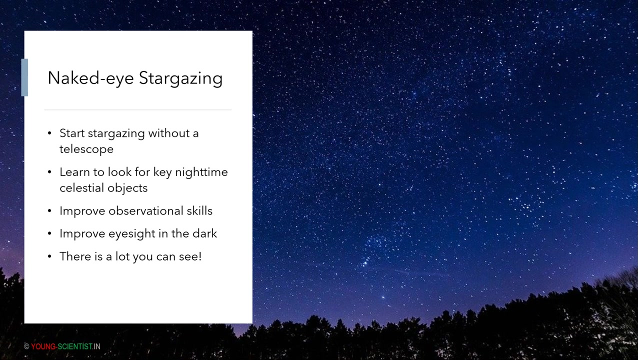 But the sky is untouchable. It's beyond our reach. Some might even say that it is eternal and even divine. Maybe that's why they point at the sky when they talk about heavens and other related stuff, Even though we now have telescopes. 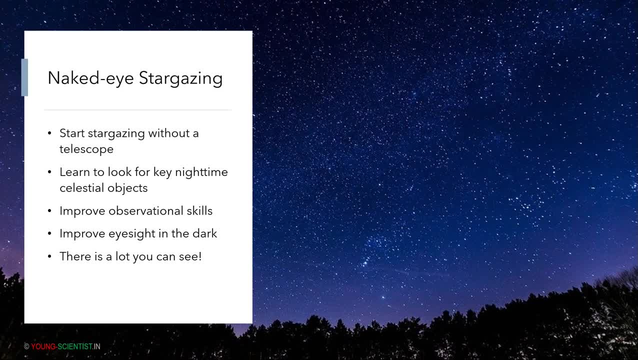 naked eye stargazing remains. This is because one can learn a lot of things from it. This practice helps us to improve our observational skills and also our eyesight. Studies have shown that people who have years of experience studying the night sky are able to see celestial objects that an inexperienced person is not able to see. 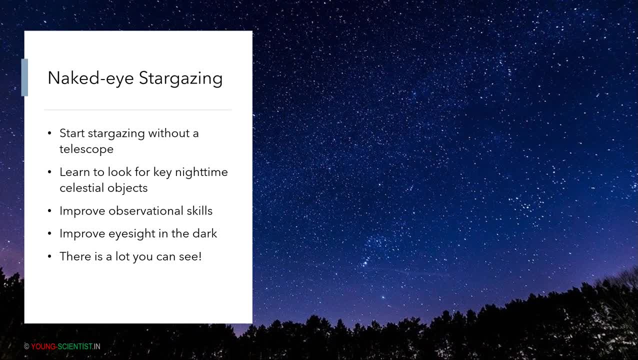 Also, even if you have a telescope, you need to know where to point it to see the things you want to see. And even without a telescope, there is a lot you can see with the naked eye. So what can we see? 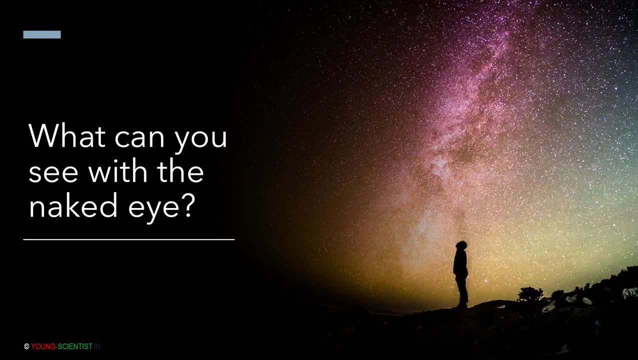 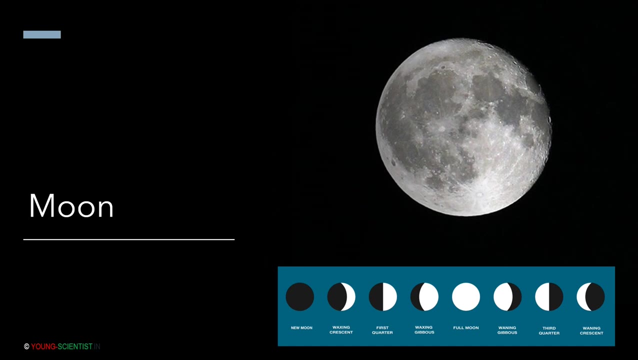 I'm sure you can think of a few different things. Why don't we start with the brightest object in the night sky? Yes, you guessed it right: The moon, Also known as Luna, Despite being the brightest object in the night sky. 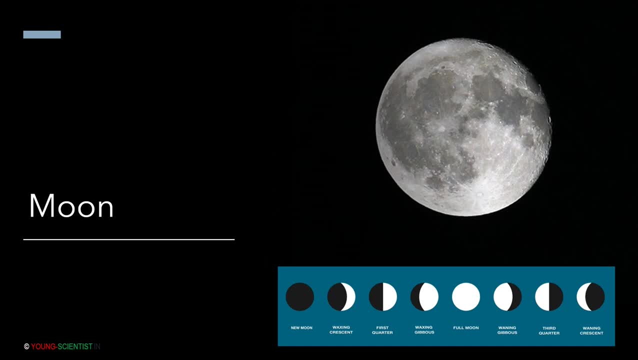 the moon does not produce its own light. It only reflects the light from the sun. In doing so, it behaves like a big mirror in the sky. In this photograph, we see the moon. We see the moon entirely. This is also known as the full moon. 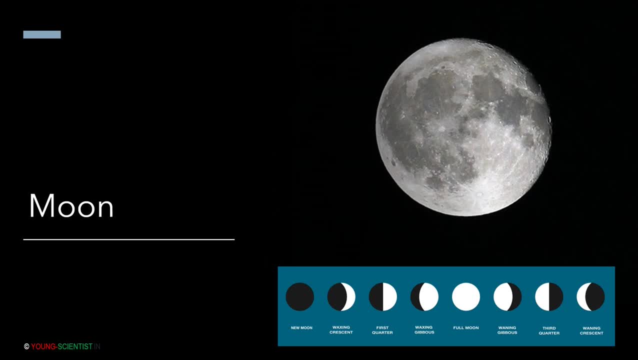 However, as days goes on, the full moon will become smaller and eventually appears to vanish. When this happens, we call it the new moon. This is because the following day, a new moon begins to appear And starts to grow until it becomes full again. 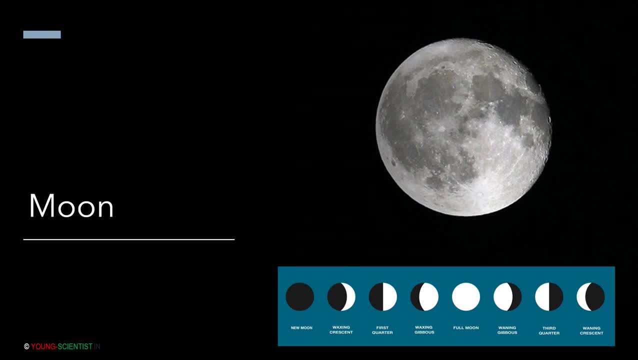 This cycle repeats itself. This cycle is also known as the lunar cycle. Many cultures have created calendars based on the lunar cycle. The moon, the full moon and the full moon start at the date of the exact month. This is because the number of days between the two full moons is always the same. 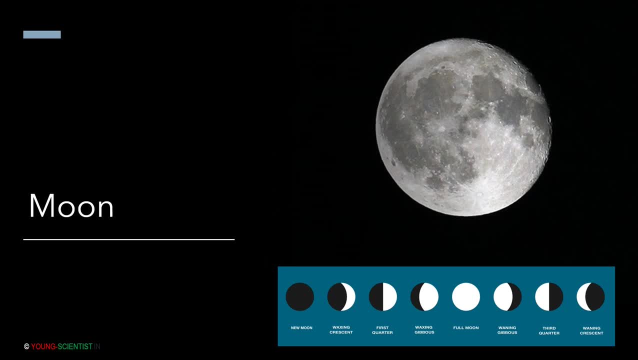 The moon alwaysliyor on the one channel instead of the two full moons. Therefore, the moon behaves like a big clock in the sky. Therefore, the moon behaves like a big clock in the sky. In order to use a clock, the moon acts as the clock. 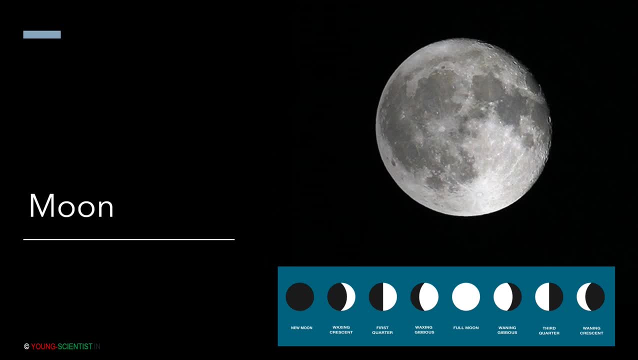 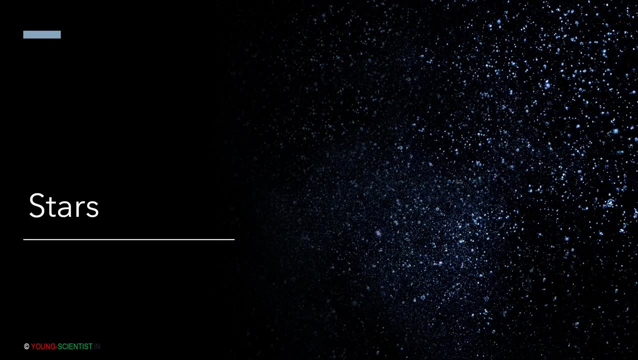 Now, what is a night sky without some? Yes Stars, Yes Stars, Yes Stars. there is a lot to be said about stars. you might know that the sun is also a star. however, the sun doesn't look like its brothers during the night-time, because the sun is much closer to us. 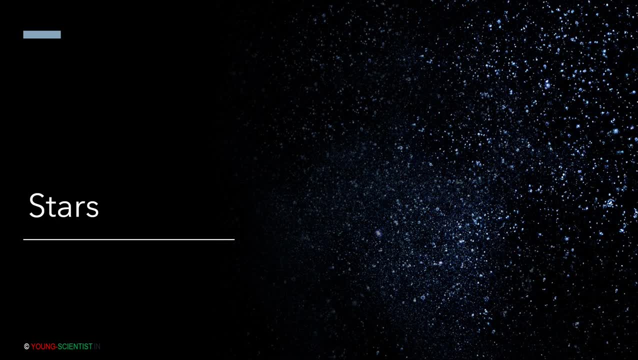 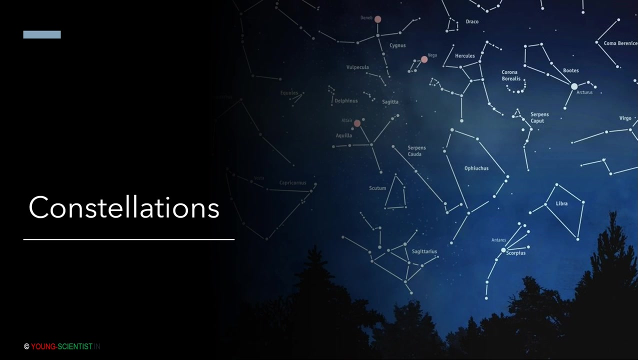 ancient humans used these stars to draw figures in the sky. yes, they connected these dots and then they saw some interesting shapes. we call these shapes as constellations. now these drawings might seem like scribbles to you, but to ancient humans they represented important objects, figures and even gods. 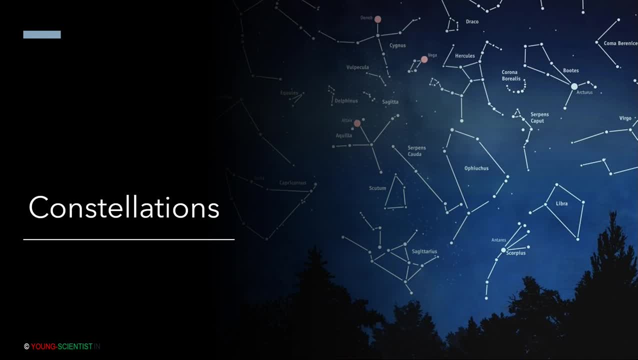 to give you an example, the constellation scorpius represents a scorpion. during the activity time, we shall try to identify a few of these constellations in the sky. depending on where you are and what time of the year it is, the constellation you find will change. 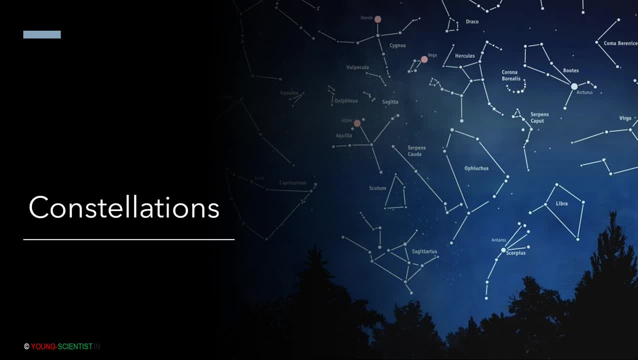 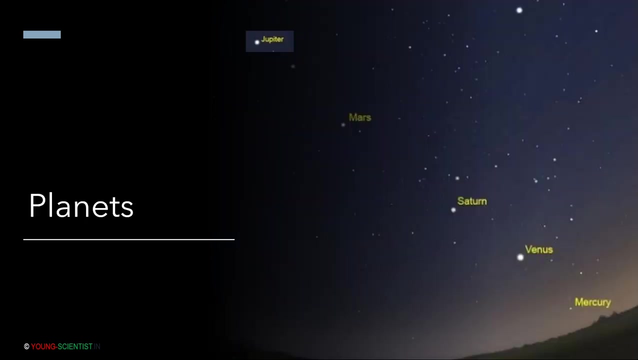 these constellations are groups of stars, and stars are famous for twinkling. yes, you might even remember a famous song about it. there are also objects like stars in the sky that do not twinkle. they are, in fact, planets. on a good night, one may be able to see up to five planets. 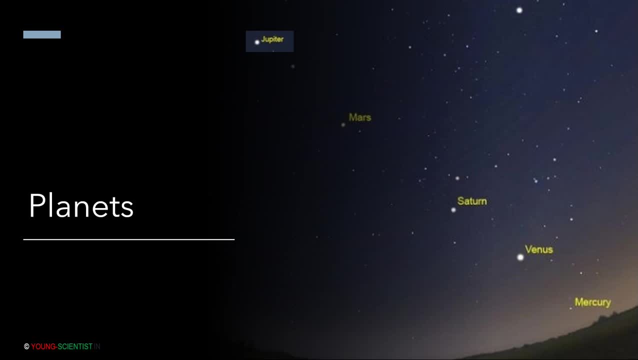 one may be able to see up to five planets without using a telescope. some of the planets are brighter than the others. the brightest planet a person can see is the venus. it is also known as the evening star or the morning star. despite the name, it is not a star, but a planet. 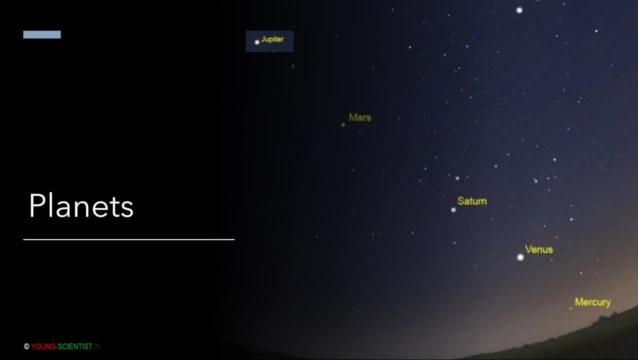 it is called so because it is the first object we can see in the sky when the sun rises or when it sets. maybe i should say it is the last star in the sky when the sun begins to rise and it is the first star in the sky when the sun sets. 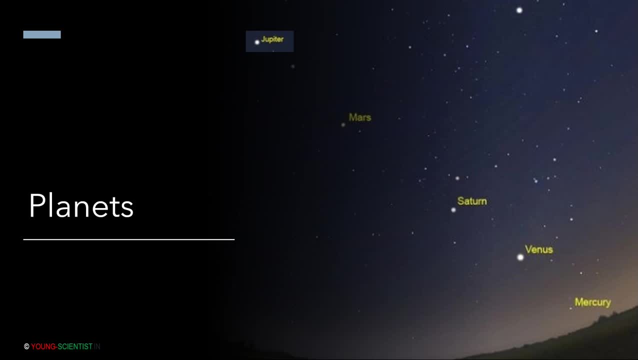 one must remember that venus is a planet and not a star. it is also the brightest object in the sky, in the night sky, after the moon, after venus. after venus, some of the brightest planets are mercury and mars. mars is quite easy to spot because it is bright red. 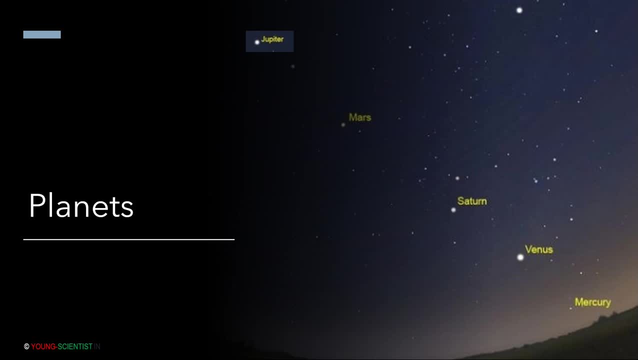 mercury is quite bright, but it is rather small and makes it difficult to spot. if you, if you are far away from the city and without light pollution, you may be able to see saturn and, if you are lucky, even jupiter. by using binoculars it becomes easier to spot saturn and jupiter. 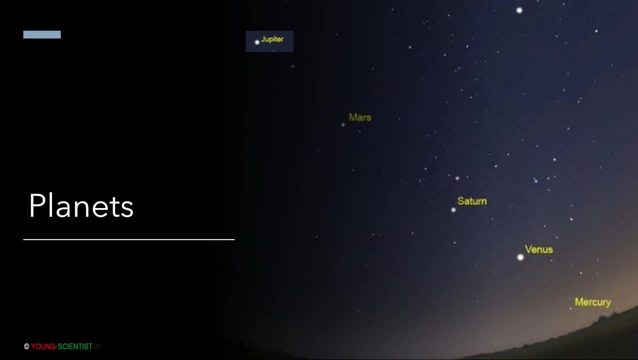 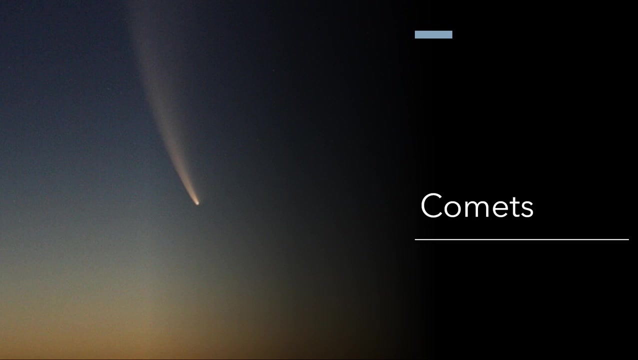 if you have a telescope, you might even be able to see the moons of saturn and jupiter. speaking of being lucky, there is a celestial object that one has to be quite lucky to see: yes, comets. one of the most famous comet is the halley's comet. 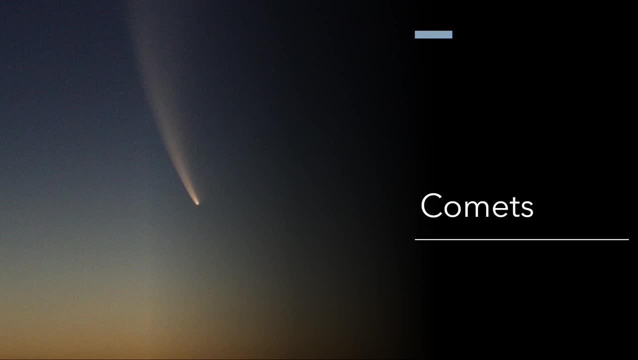 which appears in the sky only once in every 75 years. there are many superstitions associated with comets, but mostly they do not have any scientific basis. comets are visitors from beyond the solar system. they develop the tail when they become closer to the sun. we can talk more about comets later. 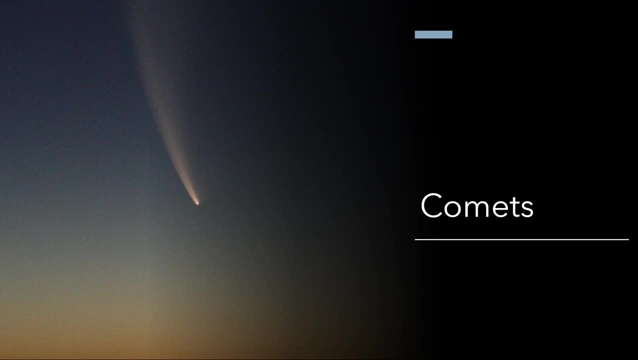 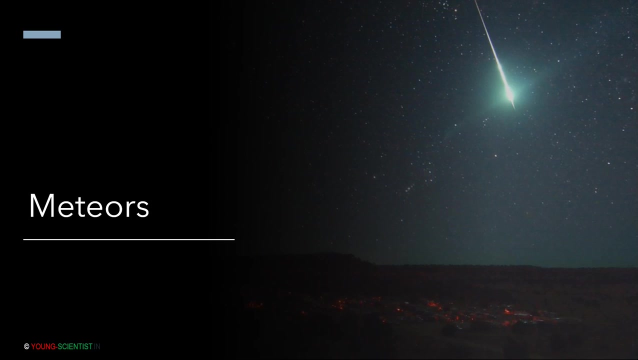 if you are interested in seeing the halley's comet, i am afraid you have to wait for another 40 years, but don't worry, you can see comet like objects if you are lucky. yes, i am talking about meteors, also known as shooting stars. despite the name, these are not stars. 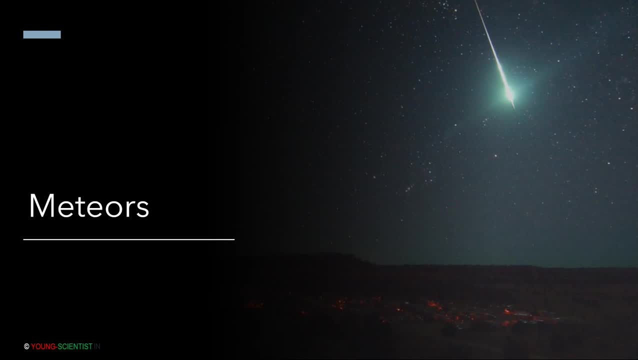 although they do look like stars and they happen to fall to the ground, they are in fact made up of small stones that find their way to the earth, and when they fall to the ground, they burn brightly in the atmosphere, creating a beautiful sight, now, if one is really lucky. 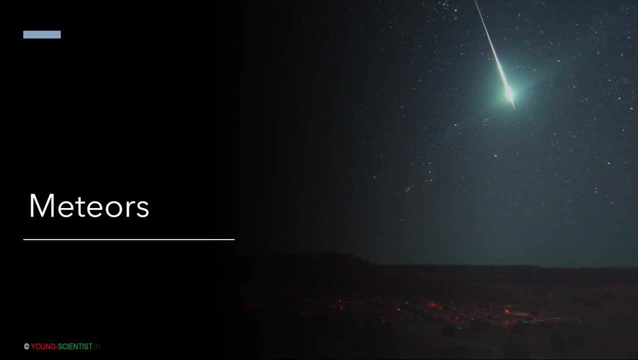 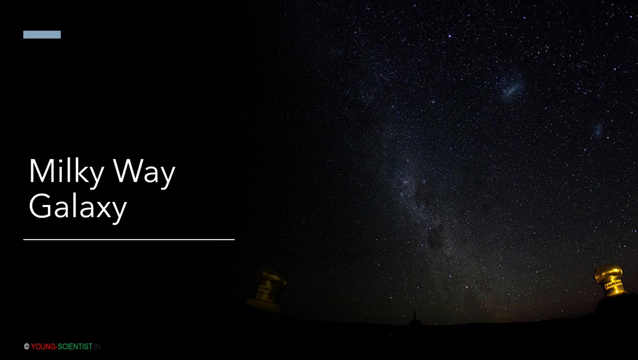 and is able to go to a place far away from cities and light pollution, you might be able to see, yes, the milky way galaxy. to be precise, you will be able to see a part of the milky way galaxy. this is because we are already in it.